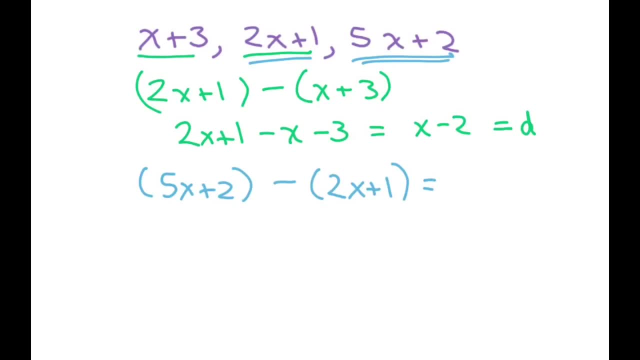 I'm going to subtract the previous term, which in this case would be 2x plus 1.. And that's going to give us 5x plus 2 minus 2x minus 1.. And that's going to give you: 3x plus 1 equals your d. 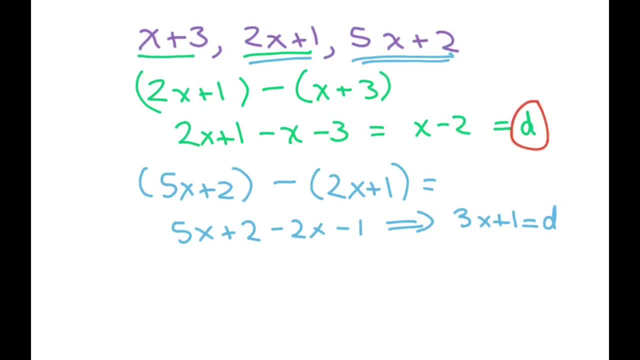 Now we have our two d's, so we have a system of linear equations. So since I have two d's, I'm going to set them equal to each other. d equals d, So we have x minus 2.. x minus 2 equals 3x plus 1.. 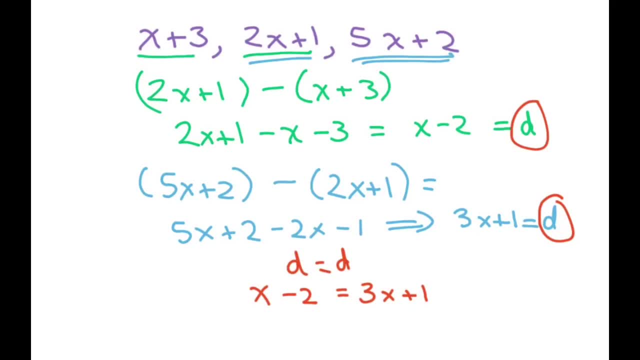 So you can solve for this, You'll get – I can move this x over here, So I get 2x equals negative 3. I just subtracted the x and subtracted the 3. So x equals negative 3 halves. 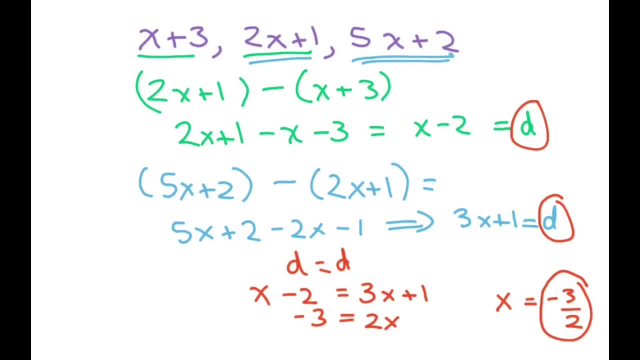 If you plug negative 3 halves into each of these x's, you will have 2x plus 1.. So that's going to give you 3x plus 1. So you can solve for this. You can also do this in consecutive terms. 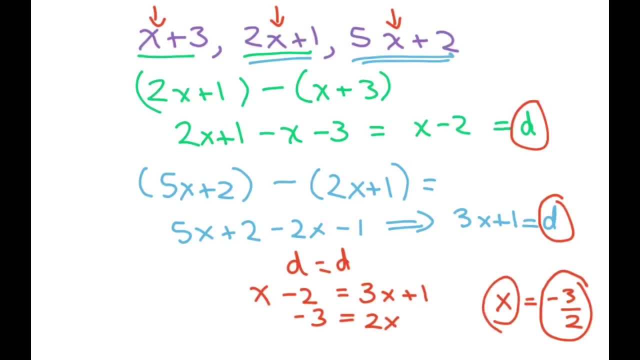 But they're just asking for x and that's all we did. Thank you, Have a nice day, Bye, bye. 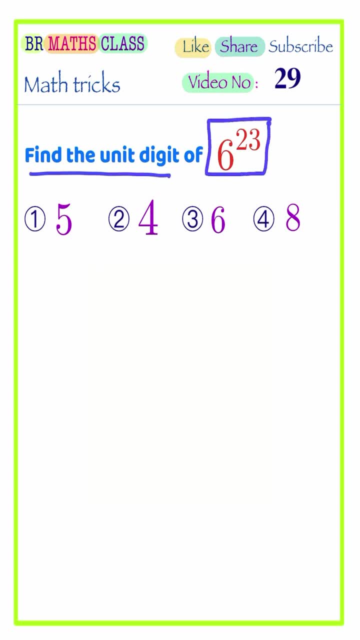 Find the unit digit of 6 power 23.. To find the unit digit of 6 power 23, there is a trick. You observe some of the 6 powers: 6 power 1 is 6,, 6 square is 36,, 6 cube is 216, like this You observe, in all these powers unit digit is 6.. So what is the unit digit of 6 power 23?? That is 6 only.